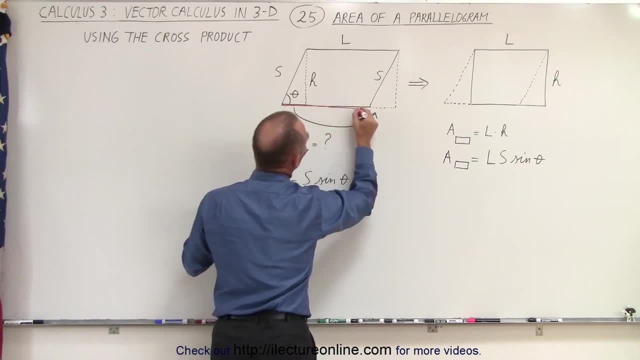 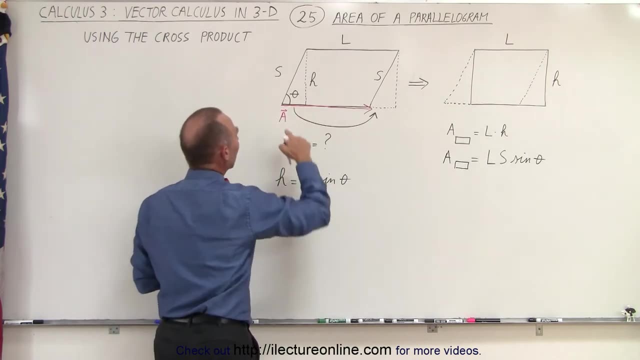 and make the length of that vector equal to the length of the parallelogram. so let's call this the vector. how about A? and then we have another vector. we draw it along the side over here. the same as the, the length of. 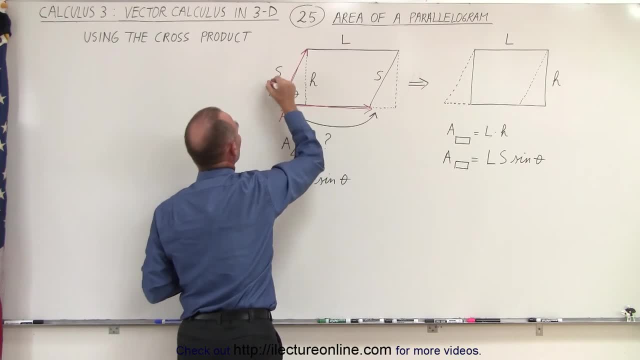 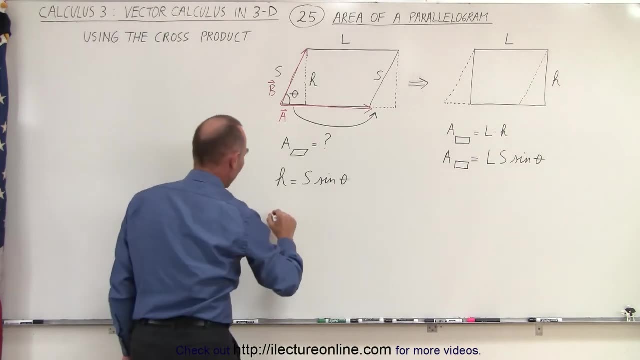 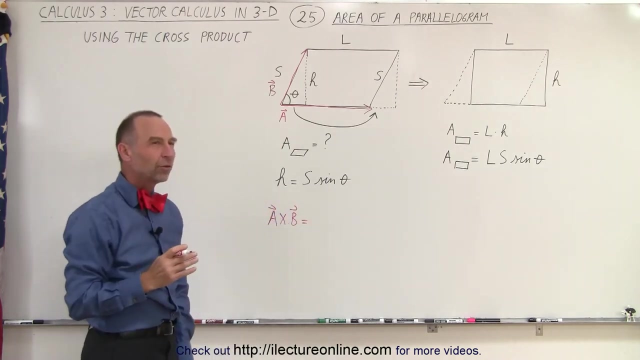 that vector will be the length of the side, and let's call that vector B. So what will we get now if we execute the cross product A cross B, so we have A cross B. well, that would be equal to well. we don't really want the resultant of the cross product, we actually want the magnitude of that. 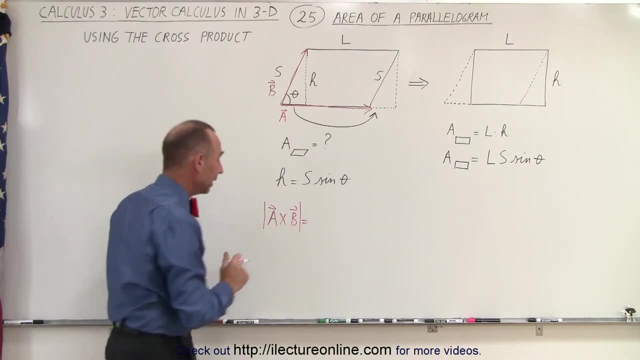 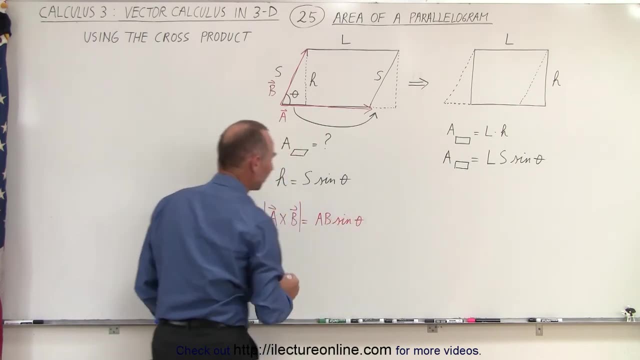 resultant. So we put absolute values, signs around it, and then what we get is that this becomes equal to the magnitude of A times the magnitude of B times the sine of the angle between the two. and notice, the sine of the angle would be the sine of this angle. 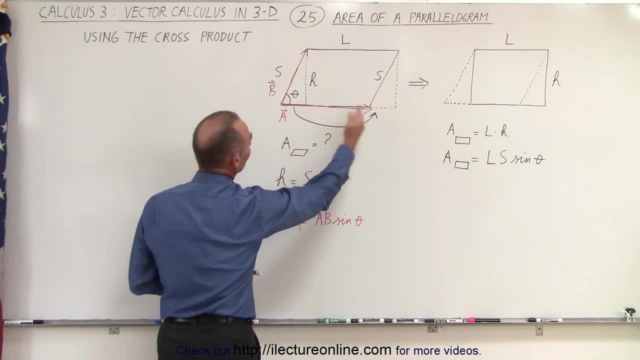 right here, sine of theta. a represents the length of this side, which is l. so then let me use black color here. so this is equal to l times b, which is the length of the side over here, which is s times the sine of theta. and of course we already know that s times the sine of theta. well, that's. 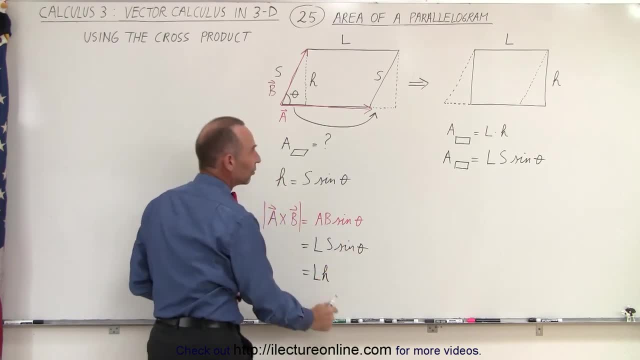 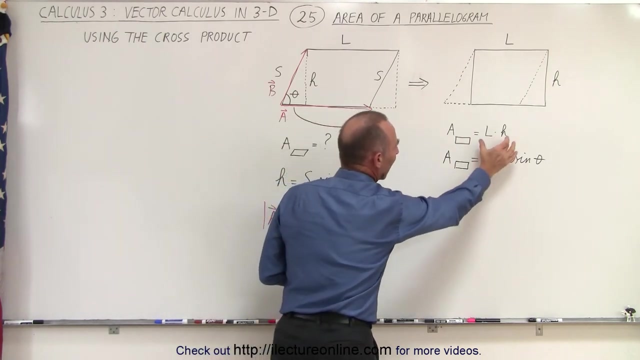 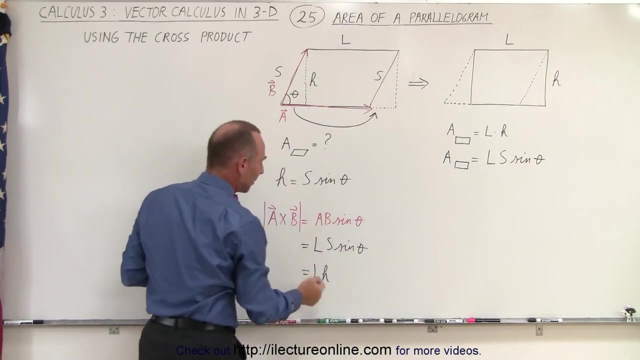 equal to h. so this is equal to l times h, which of course is equal to the area of the rectangle which represents the same area of the kitty. so here you can see that you have now the area of the rectangle, which can be written as l s sine theta, which is the same as the area of the parallelogram, and you can see that you get the. 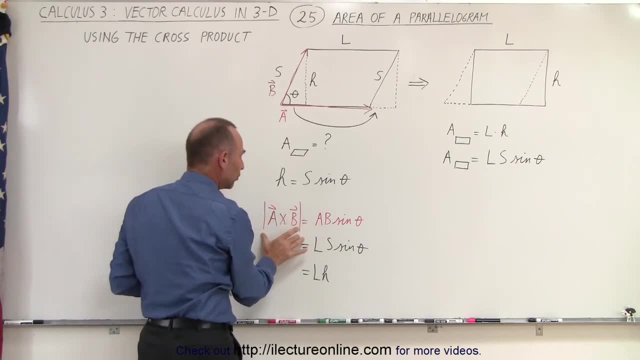 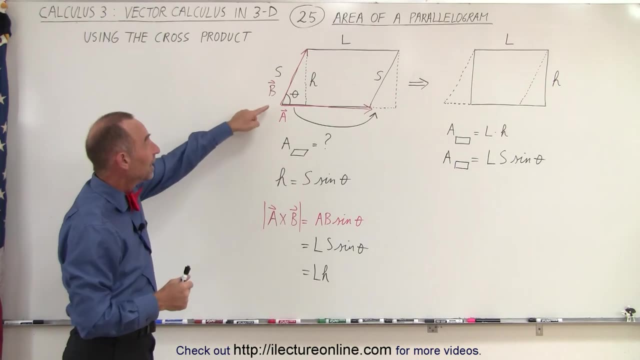 same result when you do the, when you take the magnitude of the cross product. so that's a really good way to find the area parallelogram, especially if the points of the parallelogram are positioned somewhere in three-dimensional space, And we're going to show you some real examples of that later. 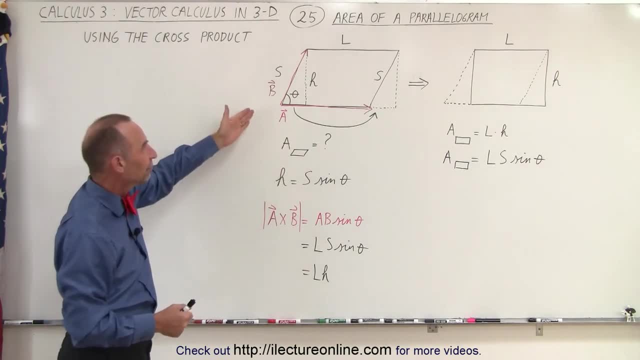 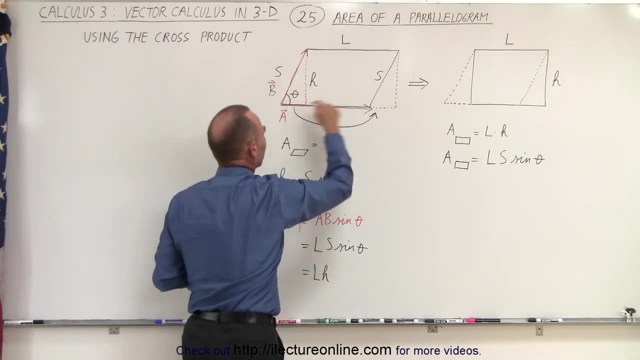 so you can see how you actually employ that, But in a simplistic, planar format. this is why, taking the cross product of two vectors representing the two sides of parallelogram, and then taking the absolute value of that, meaning, the magnitude of that,